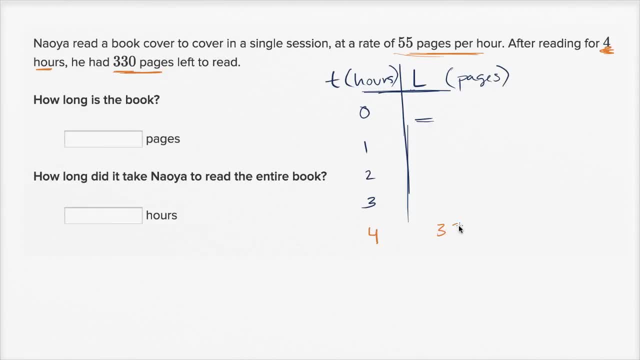 So, after four hours, he had 330 pages- 330 pages- left to read. So, based on this and the fact that he's reading at 55 pages per hour, can we back up to figure out all of this? Well, remember every hour that goes by. 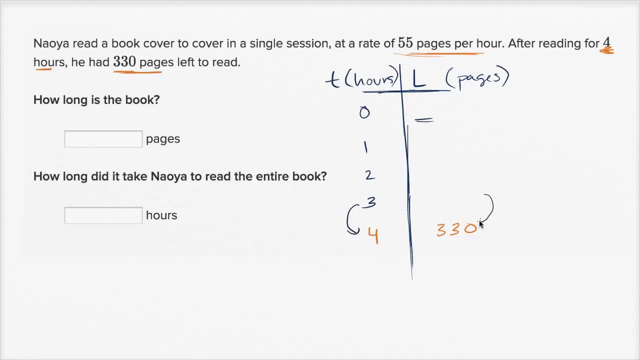 every hour that goes by, he has read 55 pages. So if he's read 55 pages, remember this: 330, this isn't how many pages he's read. this is how many he has left to read. So after every hour, 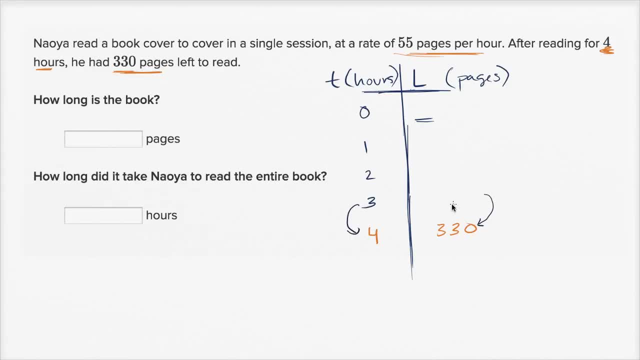 he should have 55 fewer pages to read. So at three hours he should have 55 more pages to read. So this should be: at three hours, 330 plus 55 would be 385.. Now let's see whether this makes sense. 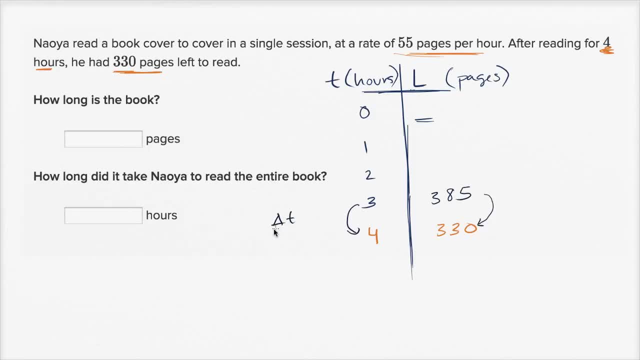 So when our change in time, this triangle is just the Greek letter, delta means change in. when our change in time is plus one plus one hour, our change in pages left to read is going to be equal to negative 55 pages. 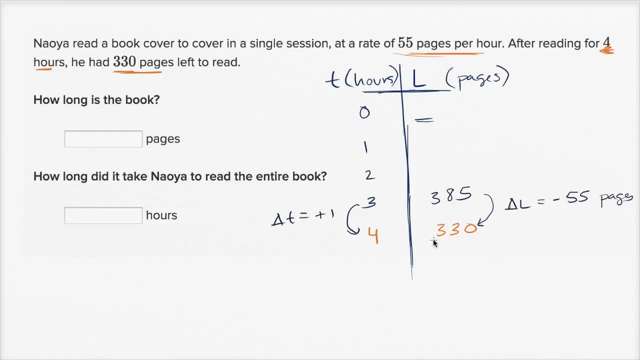 And that makes sense. The pages left to read goes down every hour. We're measuring not how much he's read, we're measuring how much he has left to read. So that should go down by 55 pages every hour, Or if we were to go backwards through time. 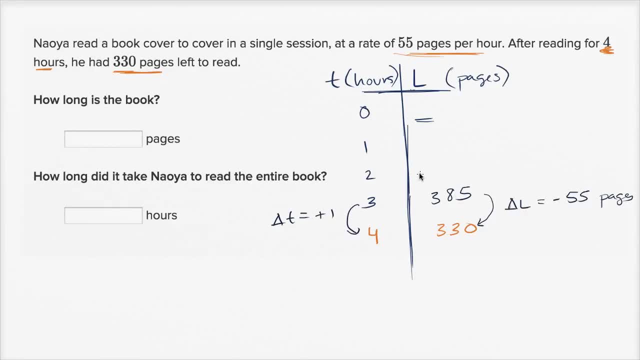 it should go up. So at two hours he should have 55 more pages to read. So what's 385 plus 55?? We'll see, 385 plus five is 390, plus 50 is 440.. So he'd have 440 pages. 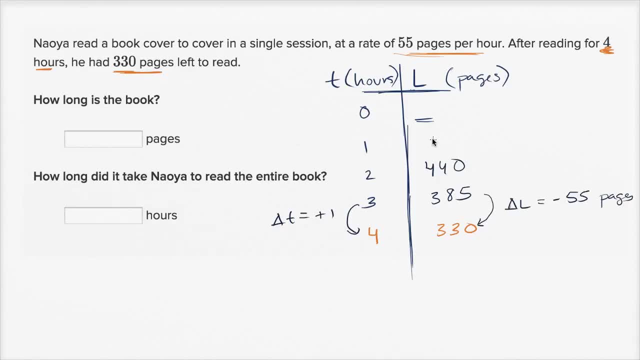 and all I did is I added 55.. And then, after reading for one hour, he would have 55 more pages than after reading for two hours. So 440 plus 55 is 495.. And then, before he started reading, or right when he started reading, 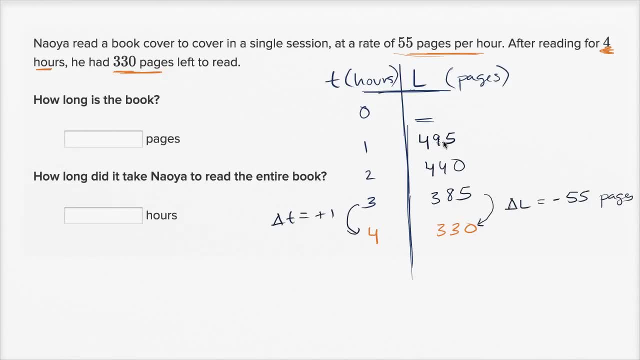 he would have had to read even 55 more pages, Because after one hour he would have read those 55 pages. So 495 plus 55 is going to be- let's see it's going to be. add five, you get to 500, plus another 50 is 550 pages. 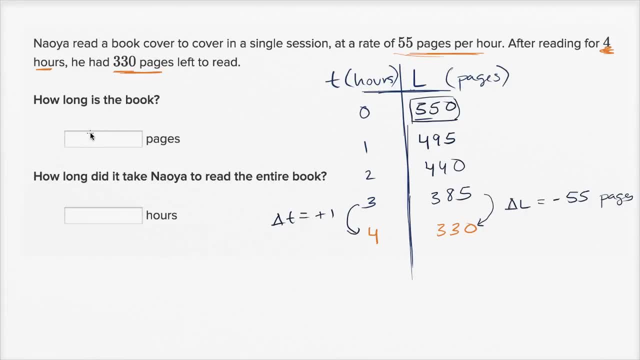 So time equals zero. he had 550 pages to read, So that's how long the book is, But how long does it take Naoya to read the entire book? Well, we could keep going. We could say: okay at the fifth hour. 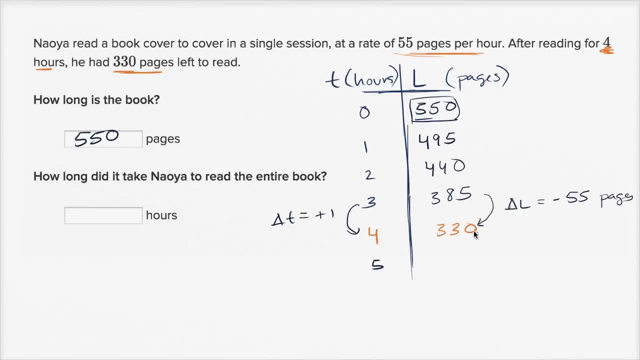 this thing's gonna go down by 55, so let's see if this goes down by 50,. if this goes down by 50, we're going to get to 280, but then if you go down five more it's gonna go to 275, and we could keep going. 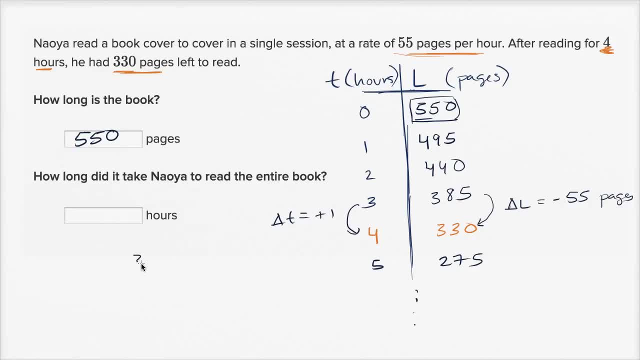 on, and, on and on. or we could just say: look, he's got 330 pages left to read and he's gonna let me write this, let me write the units down, pages. and he's reading at a rate of 55 pages per hour. 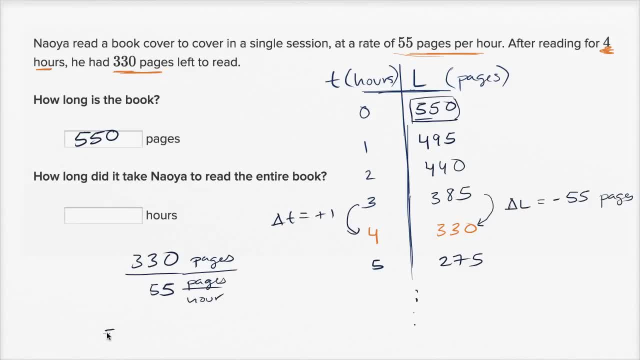 pages per hour. this is the same thing. This is going to be equal to 330 pages times one over 55 hours per hour. So if you divide by that per page, I'm dividing by something the same thing as multiplying by its reciprocal. 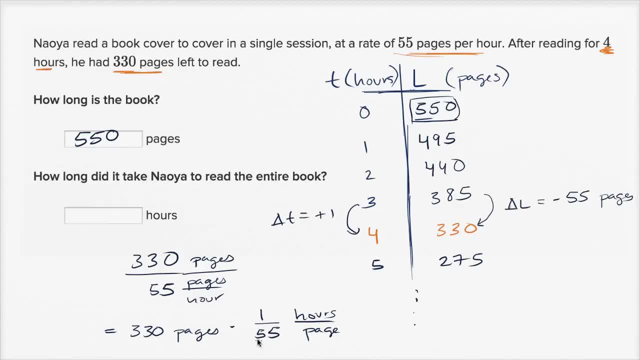 so 55 pages per hour. if you divide by that, that's the same thing as multiplying by 1. 55th of an hour per page is one way to think about it. and so what do you get The pages? cancel out pages divided by pages. 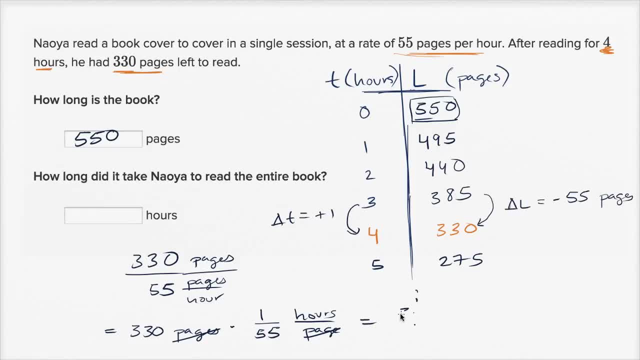 and you have 330 divided by 55 hours. 330 divided by 55 hours, and what's that going to be? Let's see: 330 divided by five is six. 300 divided by 50 is six. so this is going to be equal to six hours. 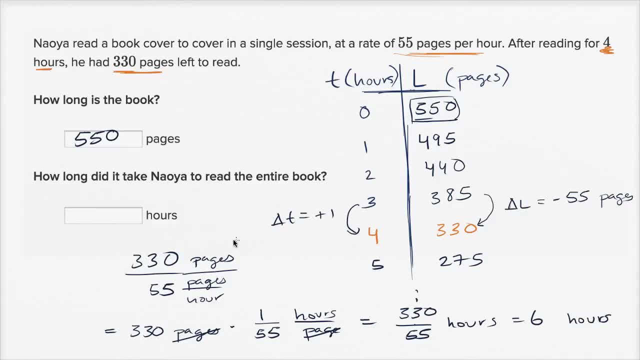 Now we have to be very careful. you might want to write six hours here, but this is six hours after this point, six hours after that point. so in total it's going to take him 10 hours. At four hours you have 330 pages left to read. 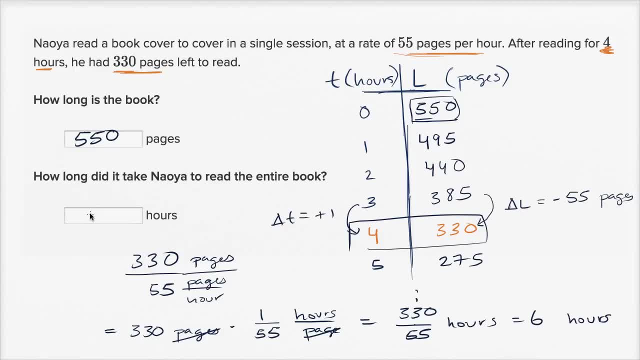 and then there's six more hours to finish those 330 pages. so it's gonna take a total of 10 hours And we could also see if this makes sense If he reads 55,, if he reads 550 pages in 10 hours. if he reads 550 pages. 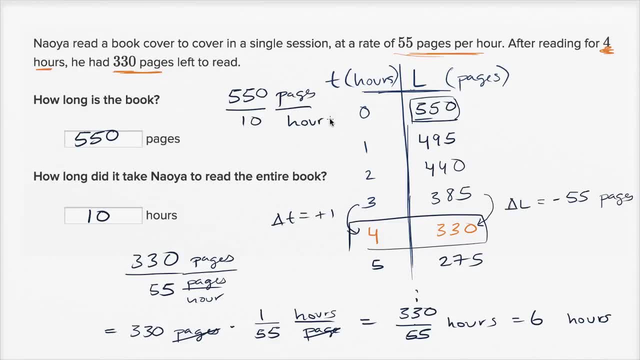 in 10 hours. in 10 hours, what's his rate of reading? Well, if it's 550 divided by 10, that's going to be the same thing as 55 pages per hour, which is consistent with what we just read. 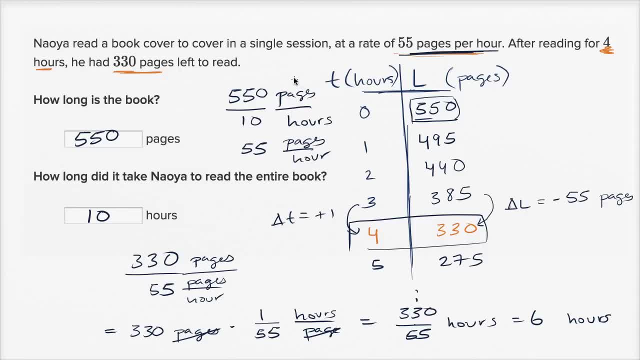 that he reads at 55 pages per hour. Now, another way that you could have tackled this. you could say: hey, this is gonna be a linear equation. if you're well versed with your linear equation, with your linear equations, you could say: 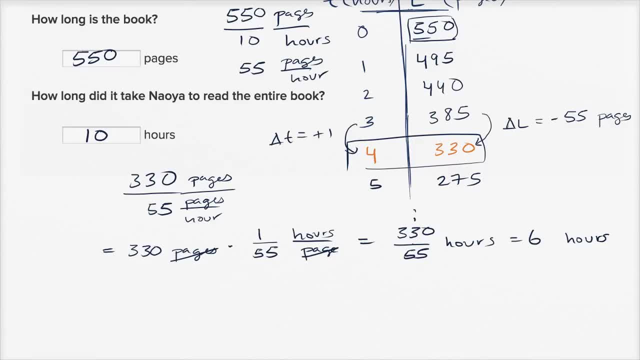 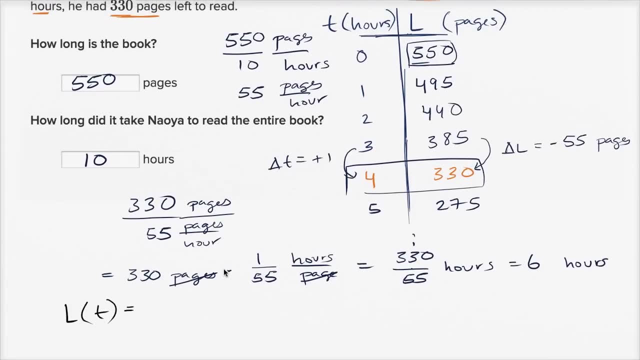 look, he's reading at a constant rate, and if we're talking about, let's say, let me just set up a function here, We could say left to read as a function of time is going to be equal to he's reading at a rate of 55 pages per hour. 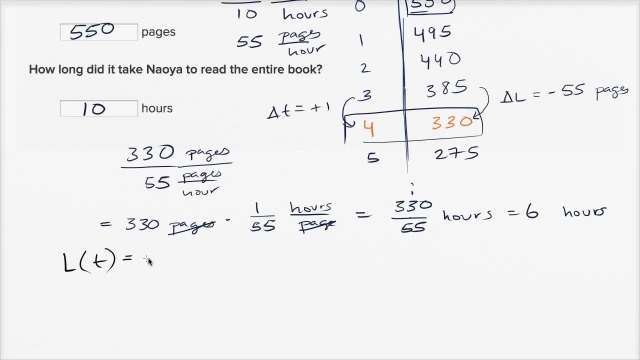 so the amount he's left to read is gonna go down by 55 pages per hour. so it's gonna go down 55 pages every hour. so you could write it like that: plus whatever the initial number of pages were, plus whatever the initial number of pages were. 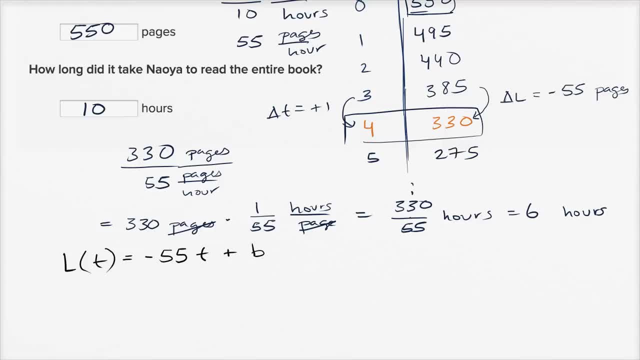 and then you could use this information right over here to solve for b. We know that when time is equal to four hours, we know that when- let me do it in that color- we know that when time is equal to four hours, that the pages left to read are 330. 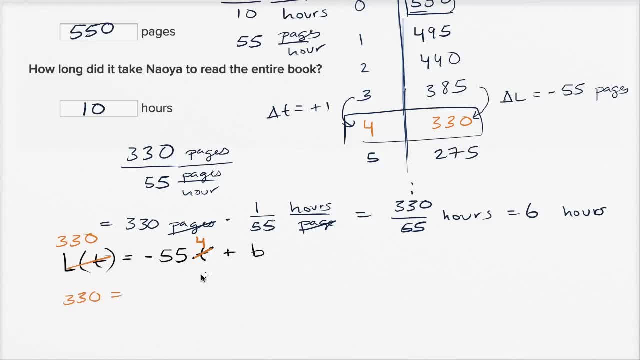 Pages left to read are 330, and so you get: 330 is equal to, let's see, negative 55 times four is negative 220.. Negative 220 plus negative, 220 plus b plus b, and then if you add 220 to both sides, 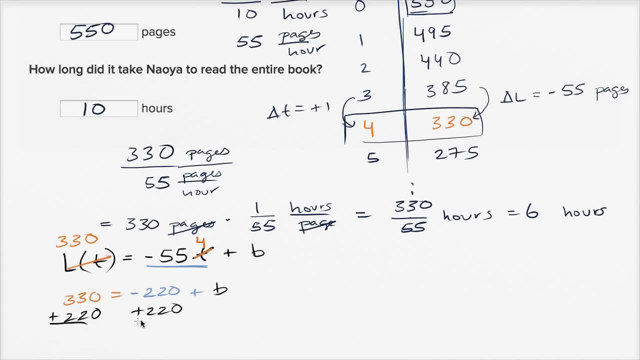 220. add 220 to both sides you're going to be left with. on this side you're gonna get. 550 is equal to these. cancel out. they add up to zero is equal to b, and so the function that describes. 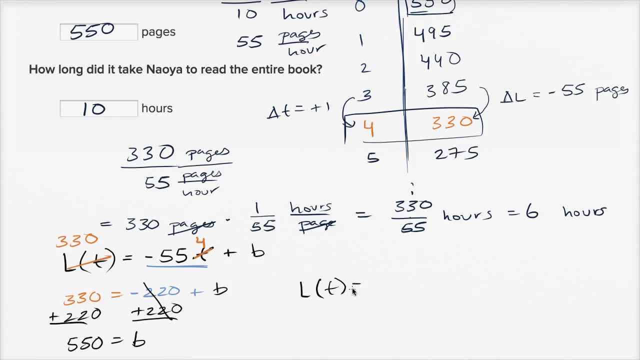 how much he has left to read. the amount he has left to read as a function of time is well, he's reading 55 pages per hour, so the amount he has left to read is gonna go down every hour. that's why we have that negative there. 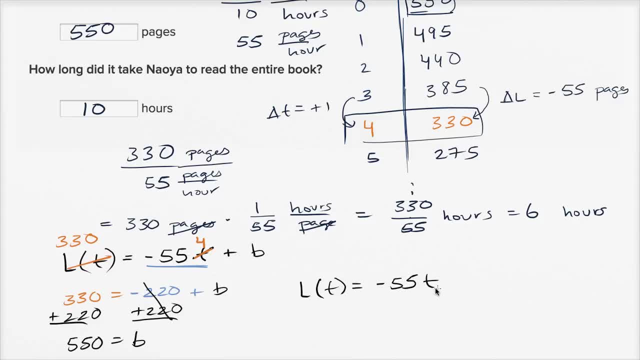 So the negative 55 pages per hour times the number of hours plus 550.. So if someone said: well, how long is the book? Well, that's going to be l of zero. That's going to be how many pages he has left to read at time zero.